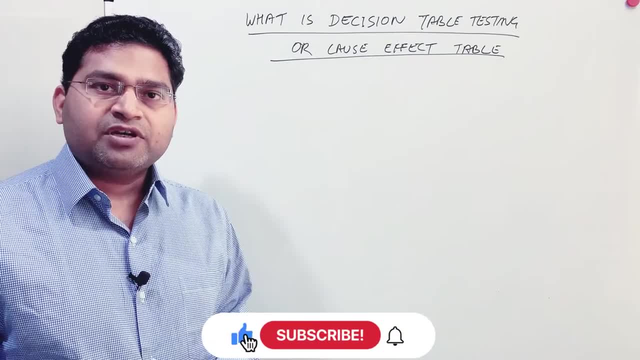 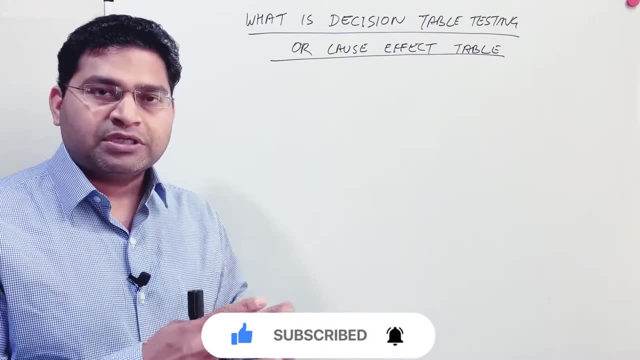 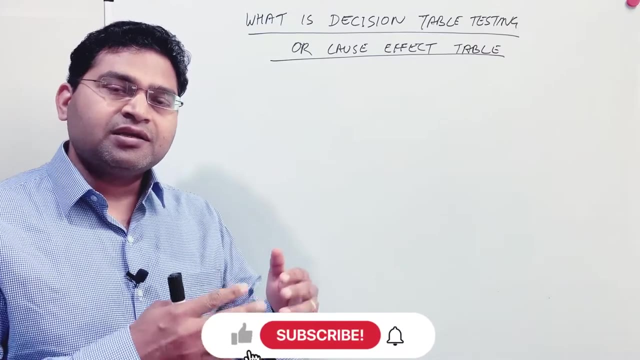 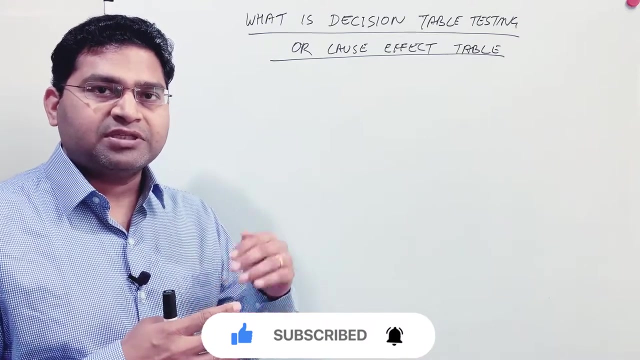 equivalence, partitioning and boundary value analysis. we have, you know, tested the boundary values or partitions of, say, for example, one rule: okay, so discount. Now, if this discount rule that is there, or discount percentage is added, or it when added with some other components, say, for example, discount percentage of an existing. 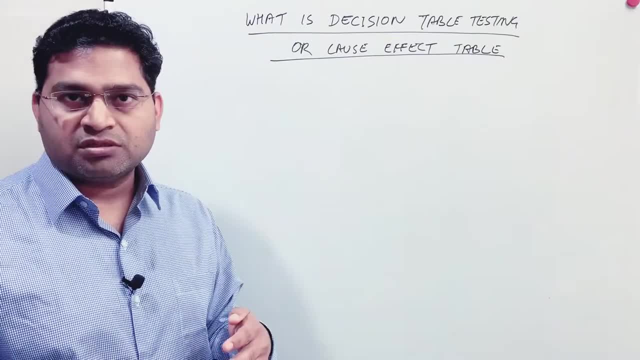 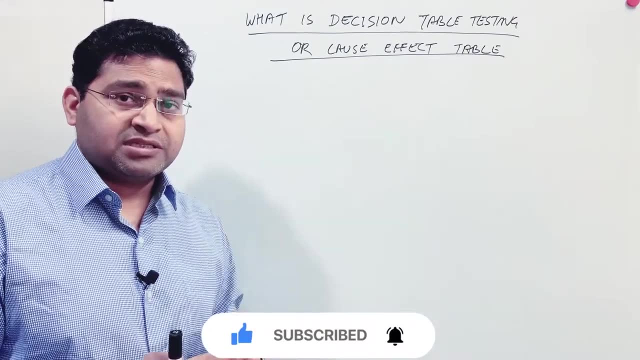 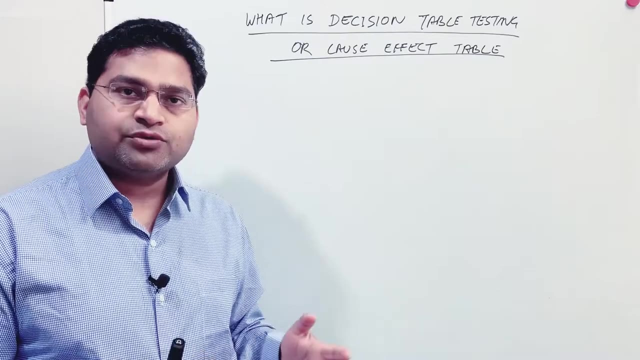 user discount percentage of a new user who registers, then that technique becomes, you know, a bit tricky to test and that's where decision table testing comes in picture. So when you have to add multiple rules and come up with the scenarios to test, we need to go ahead with the 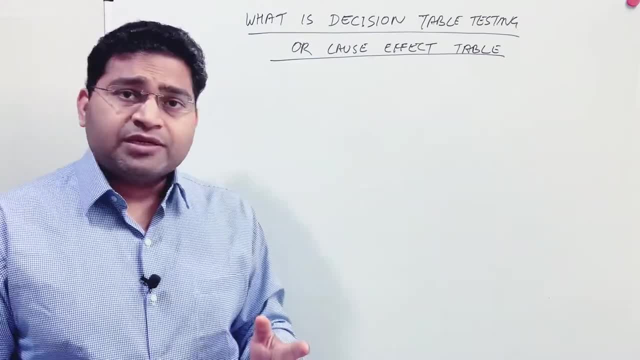 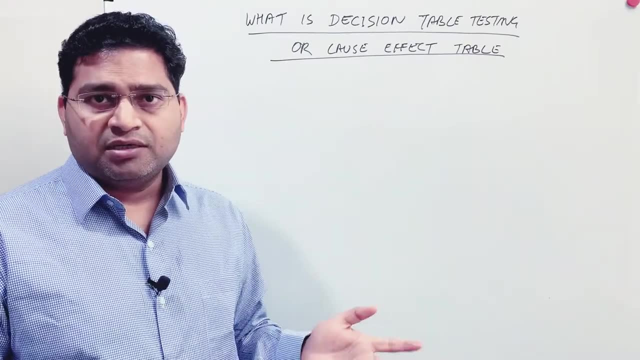 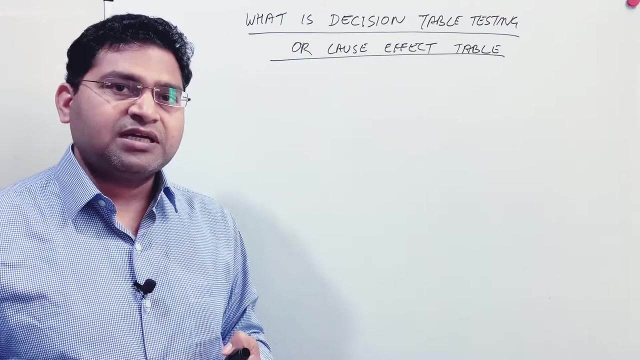 decision table testing. So I'll explain decision table testing in very simple terms so that you can correlate the same example with any of the scenarios that you can test in any of the application right. So now say, for example, there is a website which has the registration functionality and you need 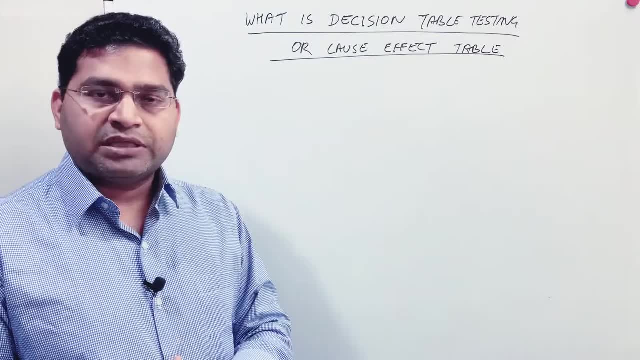 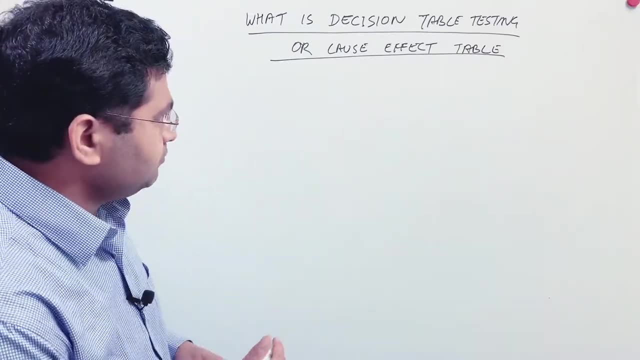 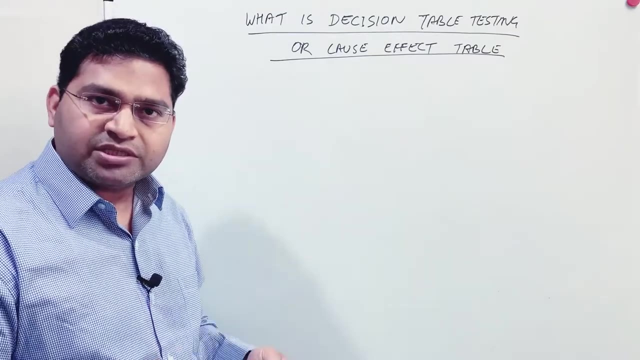 the name, email and address to register on that particular website. okay, and now you are a software tester on that particular website and you want to test. So the outcome, or basically the error message or success message of the registration, depends on these three inputs. okay, 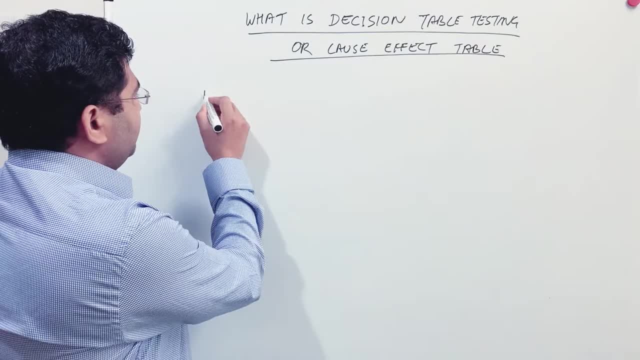 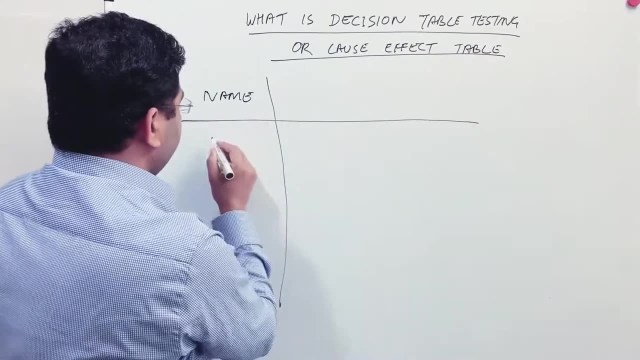 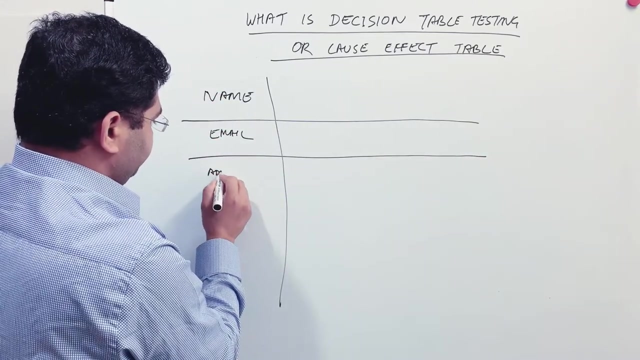 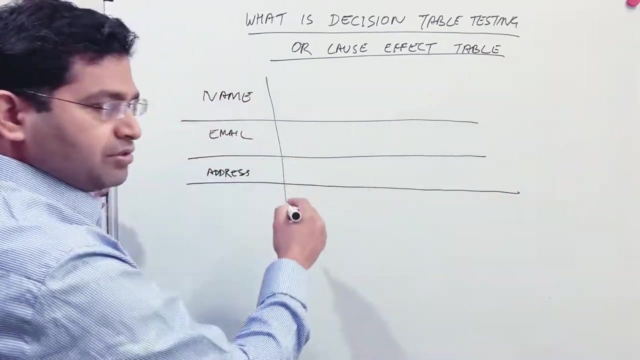 Now let's say, for example, I have name, so registration portal has name, then we have email and then we have address. So these are, say, for example, three mandatory fields that need to be entered by the customer who wants to register on the portal. okay, 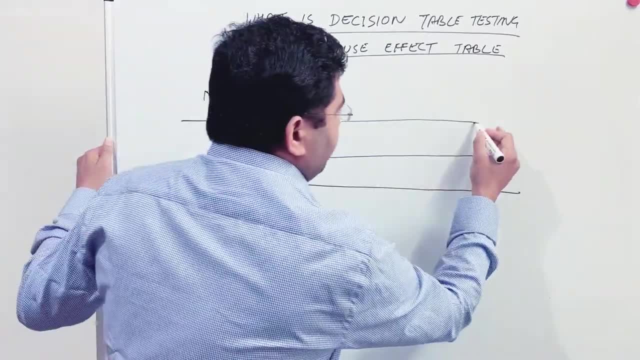 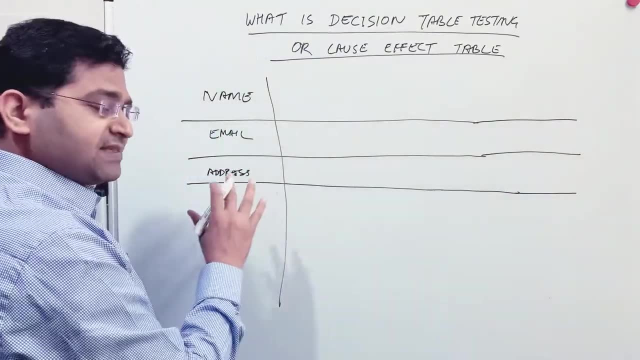 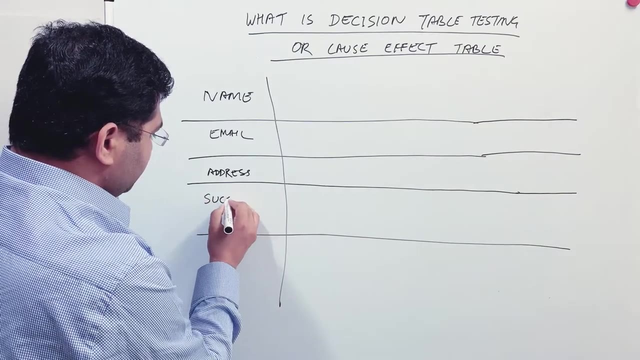 And based on the values that the customer will enter, there will be appropriate success message or error message. okay, So here at the bottom I'll write success message. Okay, Say, for example, you want to register here. Let's say, for example: 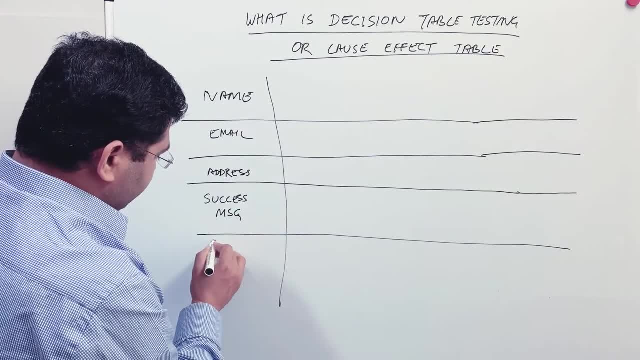 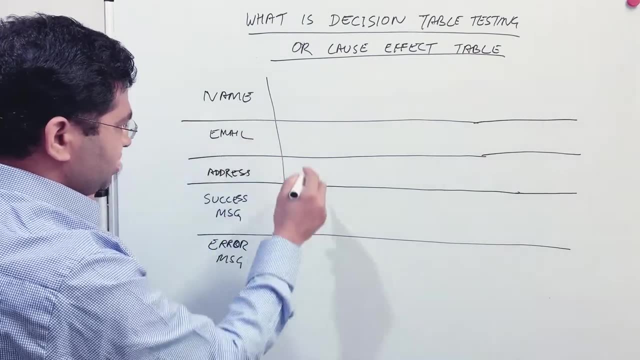 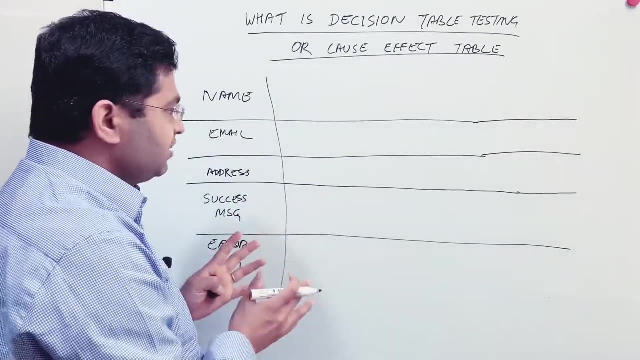 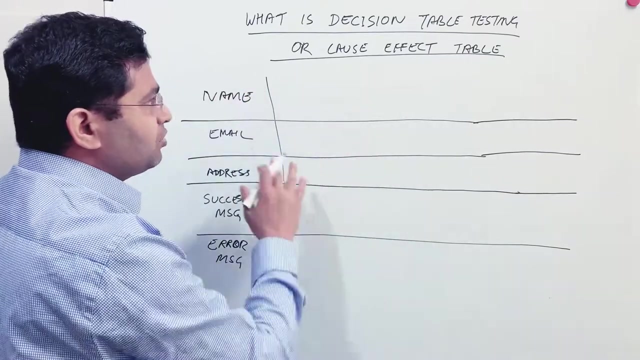 Okay, So I'll say a value, Let's say a value to test success message and error message that needs to appear in case of registration failed or successful- then how you can basically get the complete coverage and make sure that you are. you have tested all the error messages. okay, so that's where decision table or cause effect table comes. 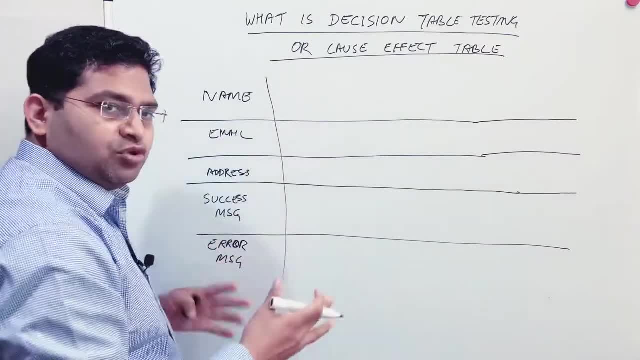 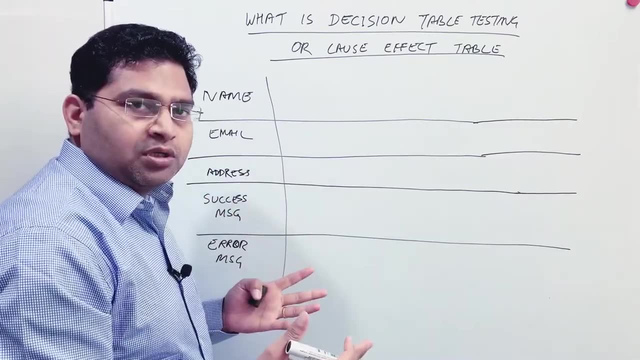 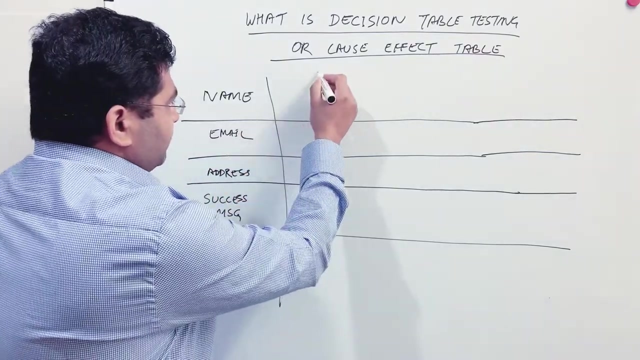 in picture now in this particular table. so mostly you will be using excel sheet to basically create this decision table. you know decision table or any tool like confluence, wherein you have the table and define these decision table right. so now say, for example, what we'll do is we'll defy divide. 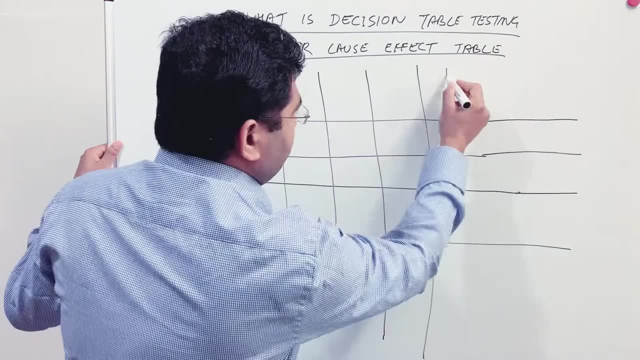 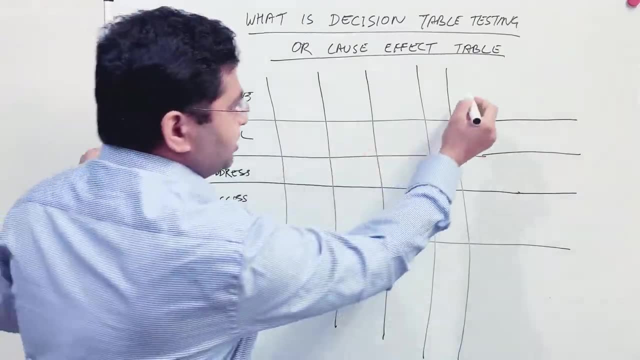 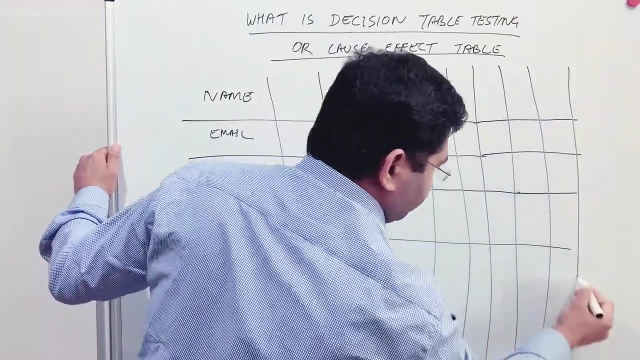 this in columns, okay, and let's see how many. so we have three inputs. so we'll be having, you know, combination of three inputs. so we'll be having, you know, combination of three inputs. so we'll be having eight combinations, right? so we'll have eight columns here. okay, all right. so one, two, three, four. 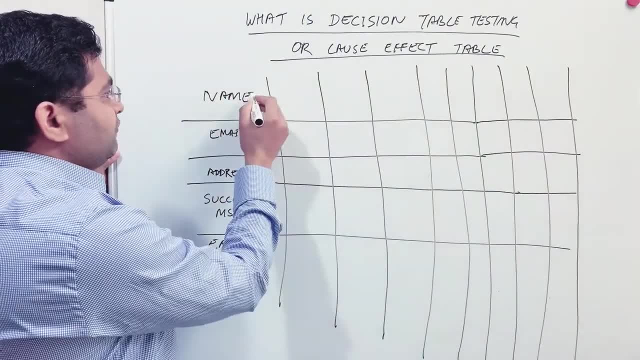 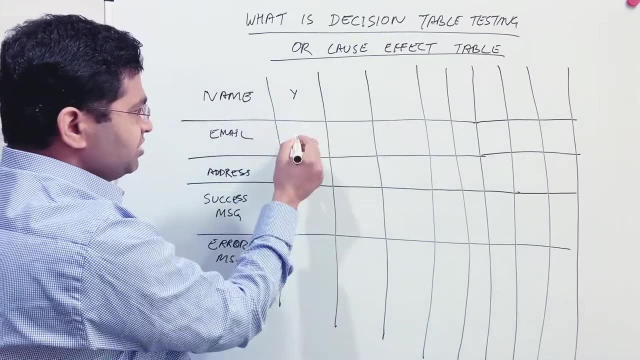 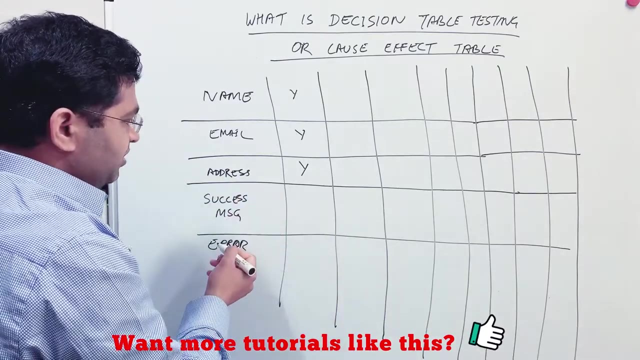 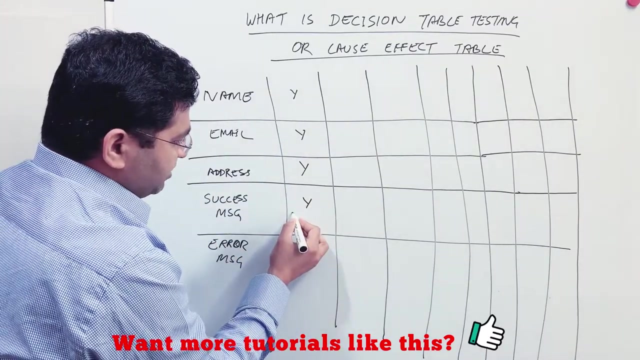 five, six, seven, eight, okay. so now say, for example, the customer has provided the name, so you can just put: yes, name is present, email is present and address is present in registration. in this particular case, what should happen? um, customer should get success message, okay, and whatever message. so you can, you know, provide the. 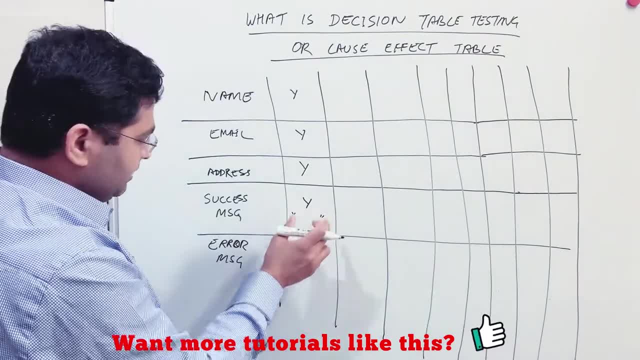 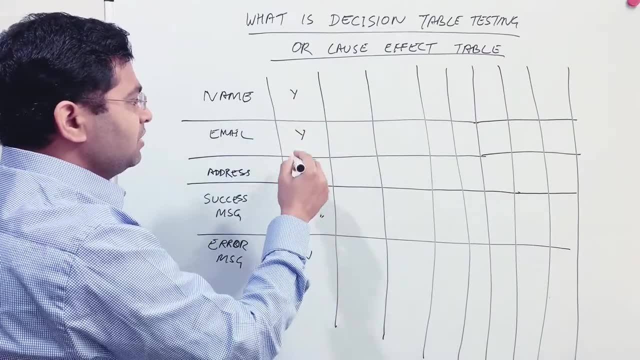 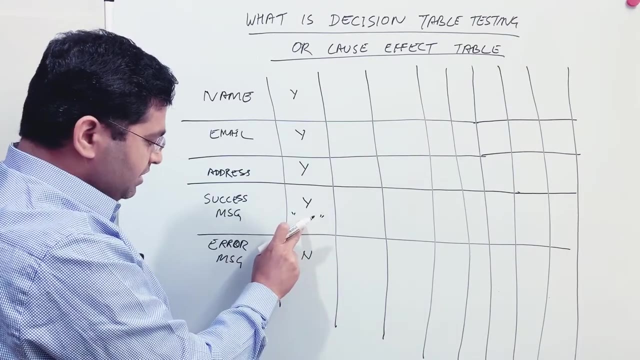 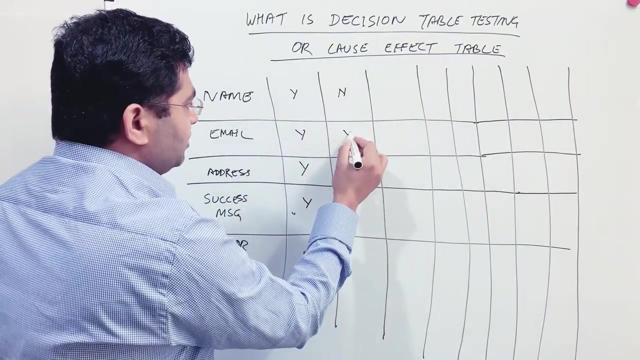 actual message that needs to be displayed in this particular column: okay, and error message should not be displayed in this particular case because all the mandatory fields that are required have been provided by the customer and the registration should be successful. okay, now if say, for example, the name, so put no there. he has provided email. he has provided address, should he? 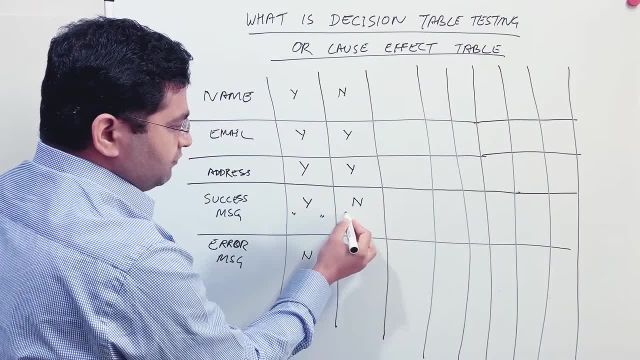 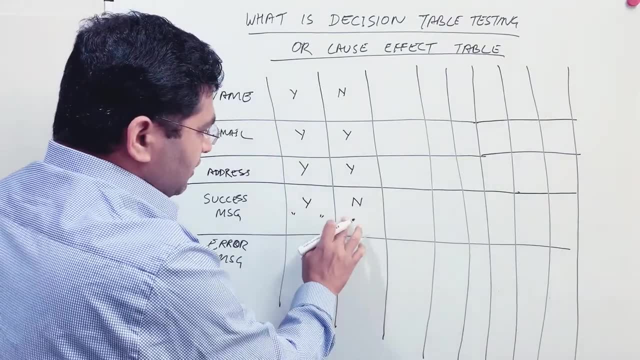 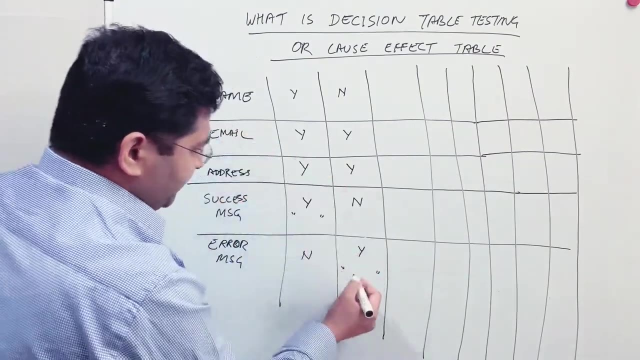 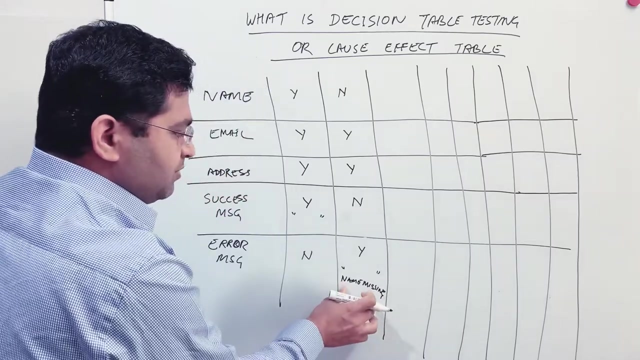 get success message. no, in this case it should fail. so you put the you know. no in the success message. there wouldn't be any success message at all. and in the error message he should get an error message and you put the specific error message, say for example: name missing. okay, now this message, the actual message. 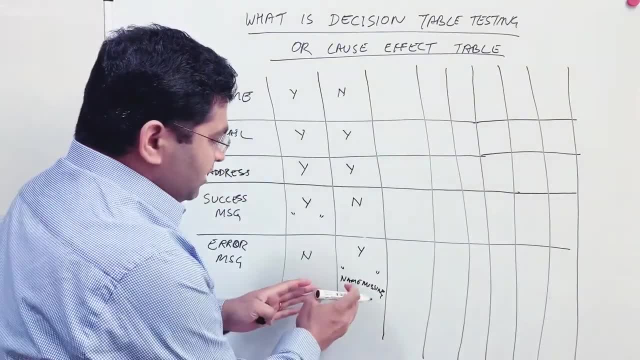 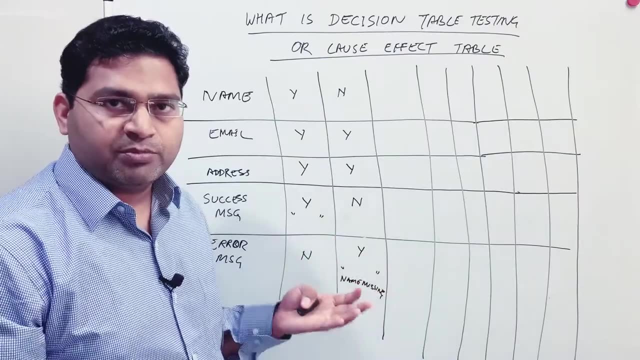 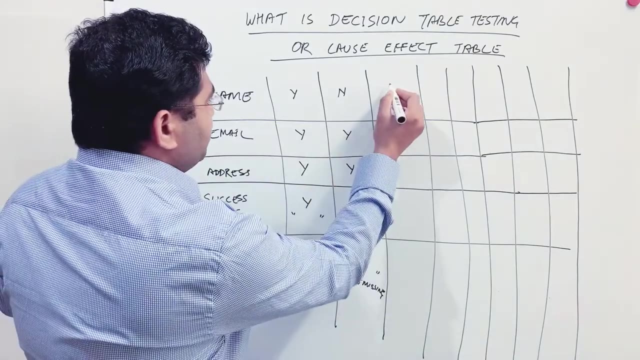 which will come from the business requirement. okay, so whatever error message needs to be displayed in this particular case, you will get it from the actual business analyst or whosoever will be providing you the requirement. so you simply copy that. you know. error message here. now name is present. or say: 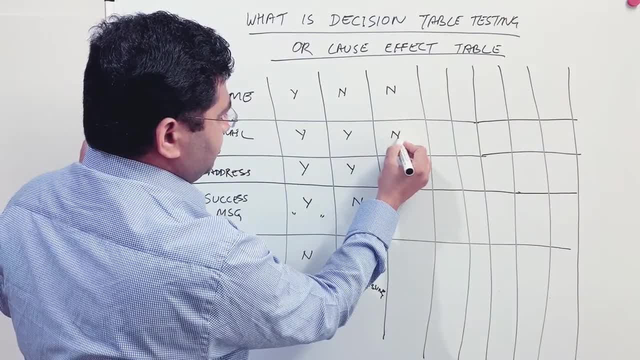 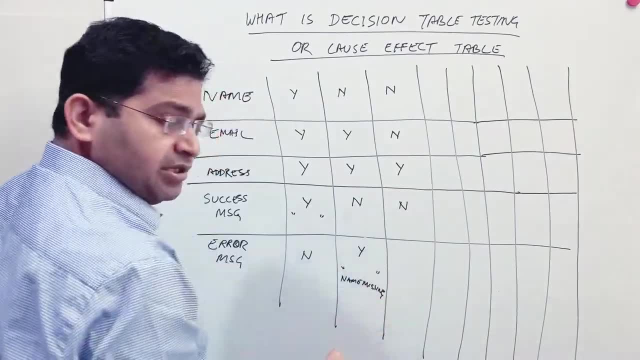 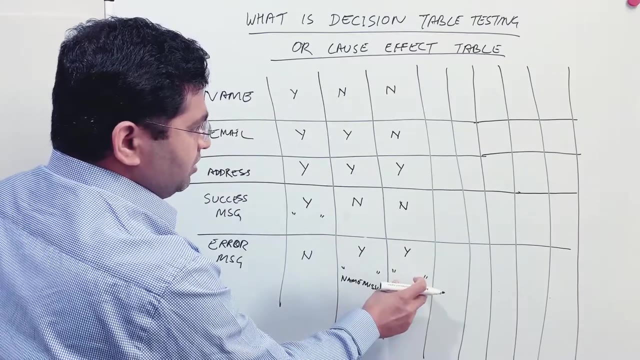 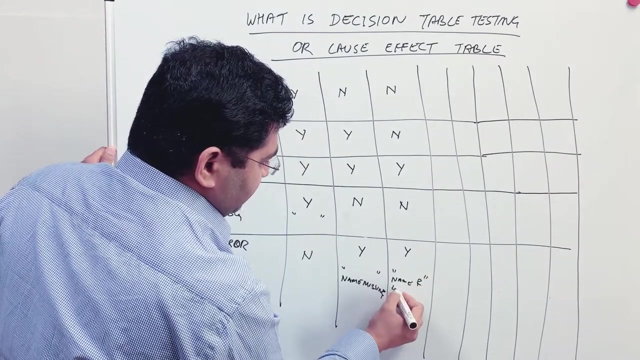 for example, name is not present, email is not present and address is present. okay, then success message should not be displayed and error message should be displayed. and what exact message should be displayed will be displayed here. okay, so in this case say, for example, name and email missing, okay, so whatever error message needs to be, 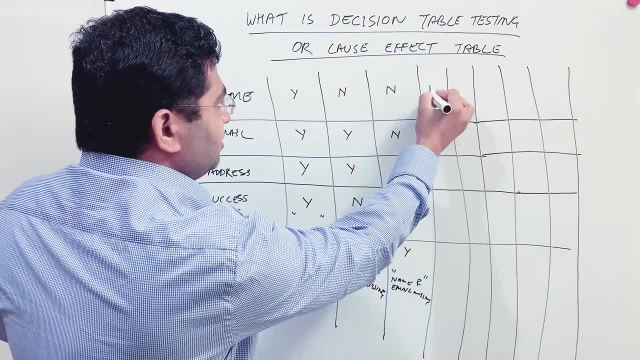 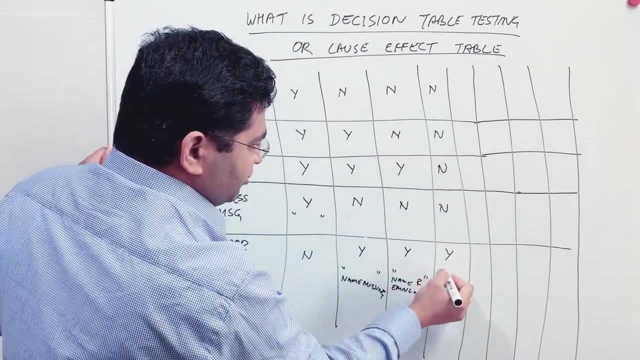 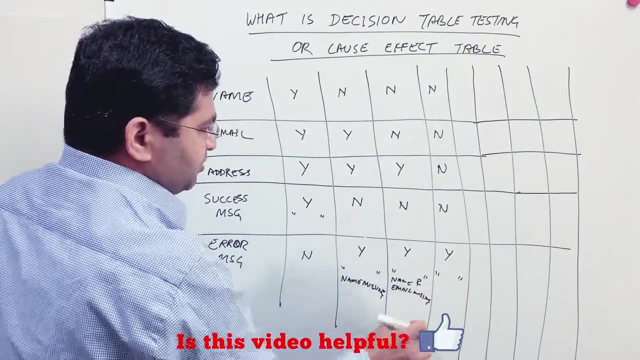 displayed in this case, you just put it here. similarly, if nothing is entered at all. so success message: no, error message yes, and whatever error message needs to be displayed- name, email and address is missing. so if a customer hasn't provided any of these details and clicked on register button or sign up button, he 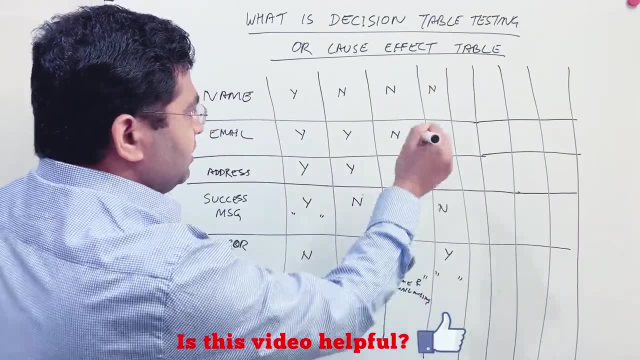 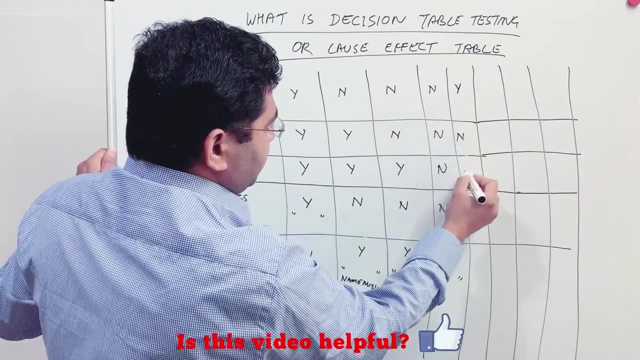 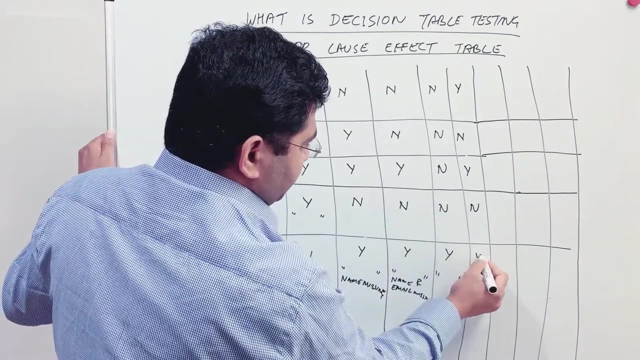 should get this particular error message okay. similarly, if say, for example, name is there, there's no email store is missing, whatever error message is displayed, it should not be done authors where this error will be displayed. you know this email is there, this error here. you know that is one message. if the question i am asking for. 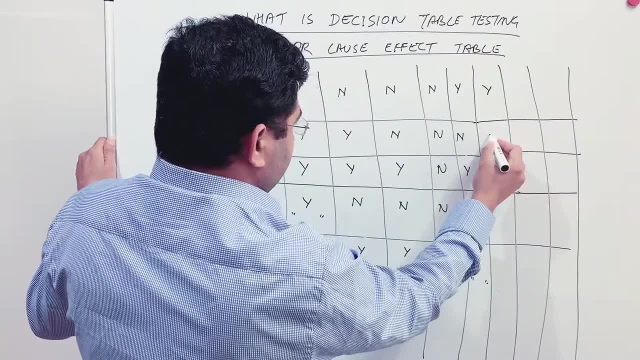 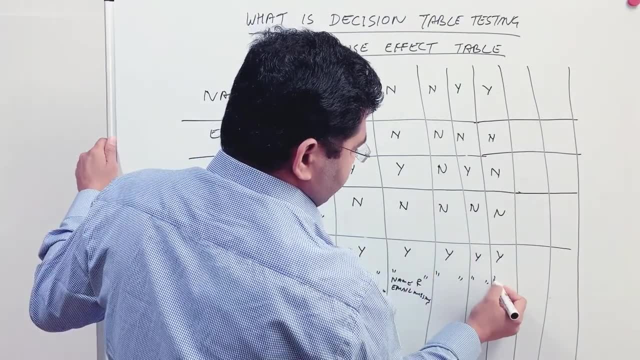 any other error messages now? if i skip this, then there will be another one here, correct? so thank you so far, this interview is for today. i have wearing glasses and いわcell rewarded you with so many feedback- amazing message. let me get back to the shop and wait a minute. so one more question, which is: what are the everywhere features are there are recipes. 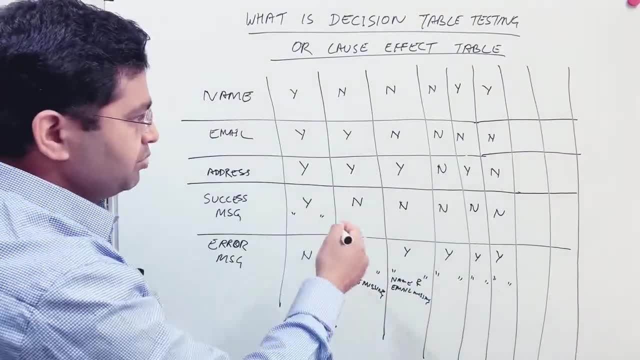 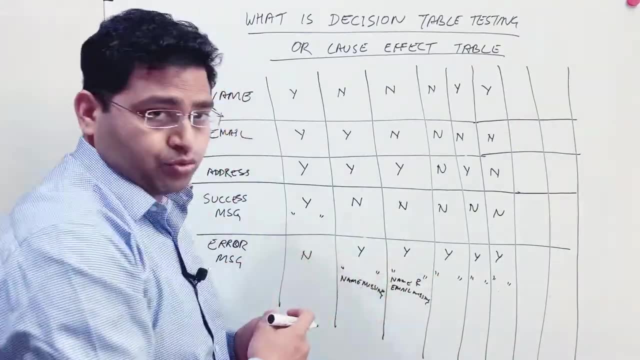 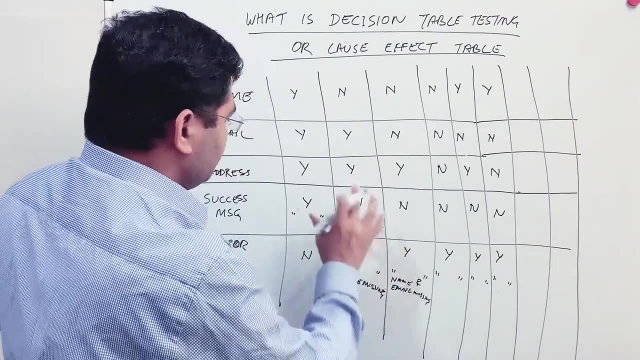 so you just continue this process unless you have covered all the error messages, different error messages that need to be displayed to the customer. okay, so if say, for example, in this particular case there are different error messages that need to be displayed if any of the value is not present, you put the specific. 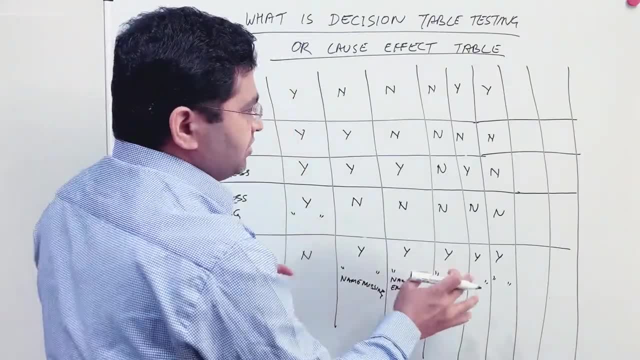 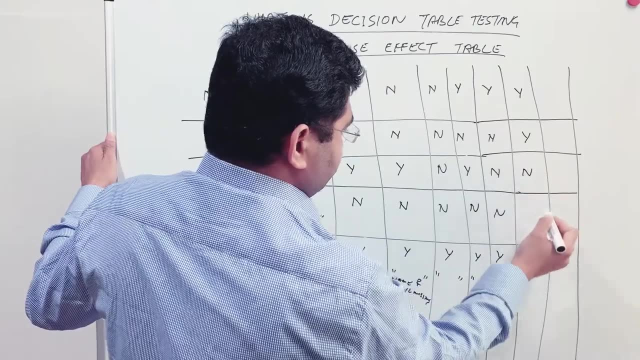 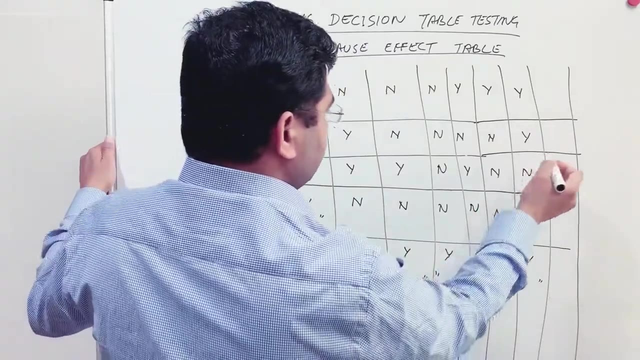 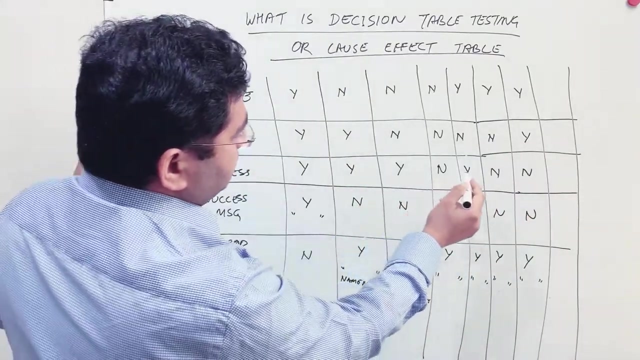 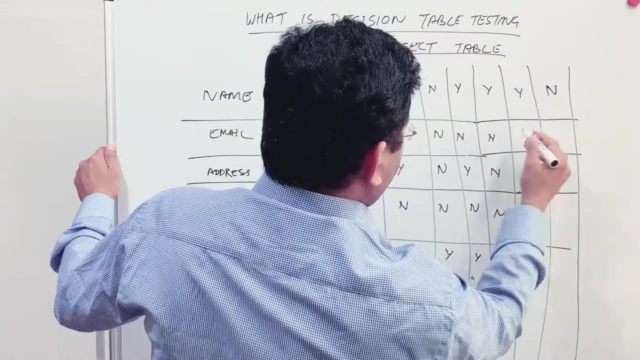 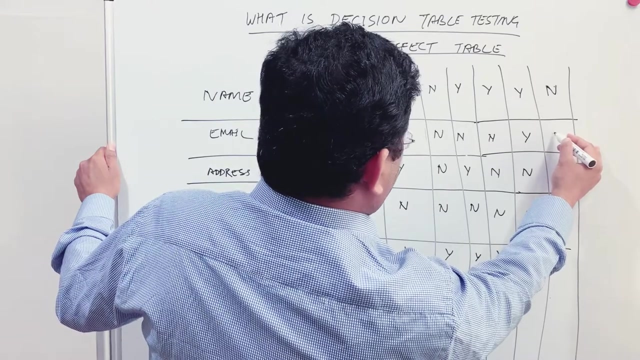 error message in each of the case there. okay, now this is present, this is present and address is not present. so no error message, no success message, error message and the exact error message. all right, then what is left? so we have? so here, we have no, and so name is missing and email is present and we have address present, our 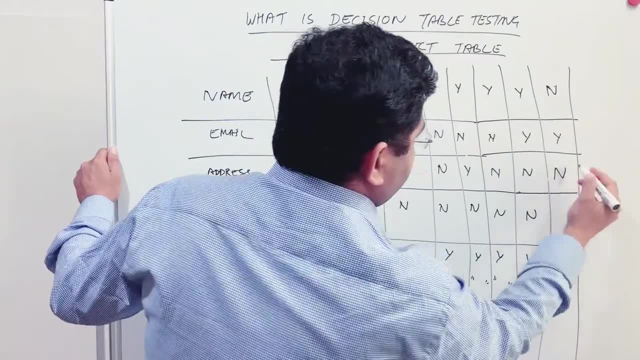 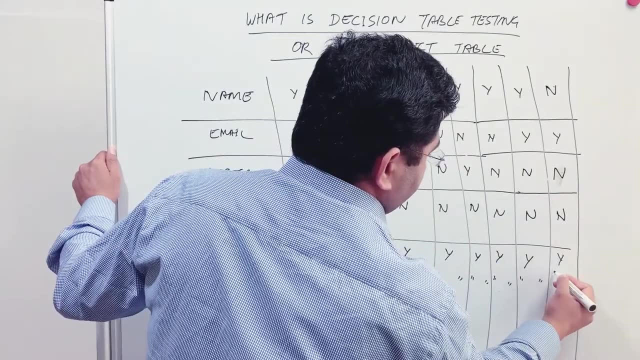 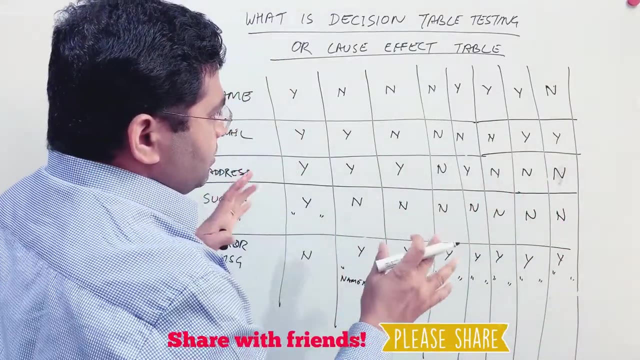 address is missing. okay, so it covers so. so, for example, this is the case, then that particular case: success message should not be displayed, error message will be displayed and error message will display something: email is missing. okay, so now, if you see that in this particular case, you know email is. 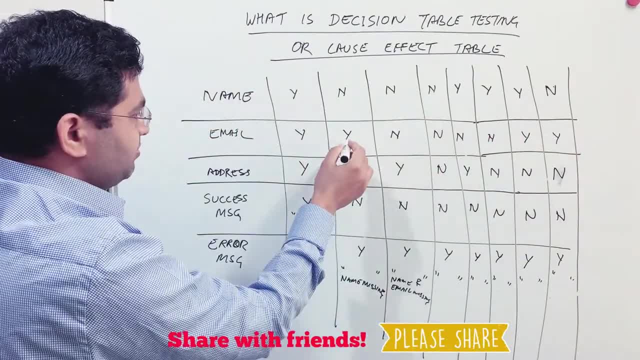 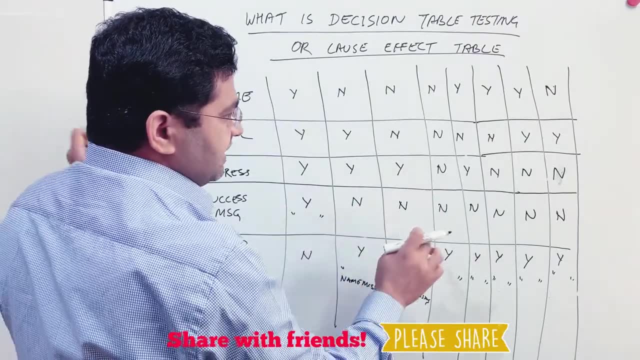 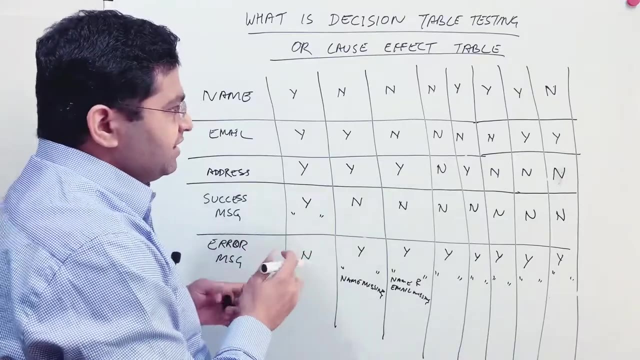 missing. here, you know, we have say, for example, separate message for email and address is missing. here, address is missing. and in this case, if there are separate error messages that need to be displayed in each of these scenarios once the values are, you know, missing, then you have this decision table. 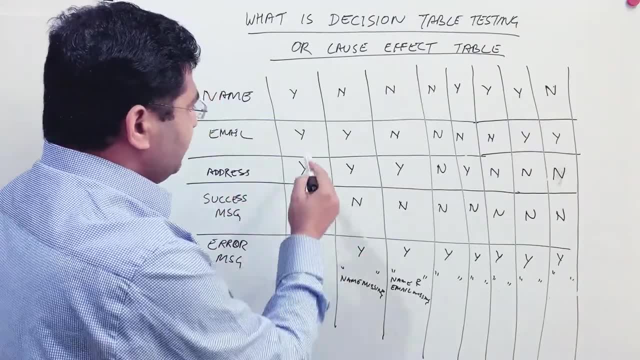 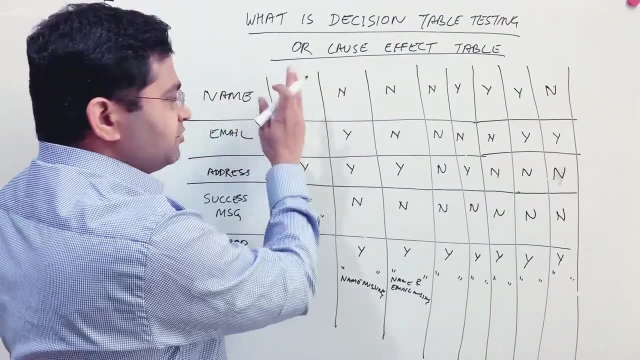 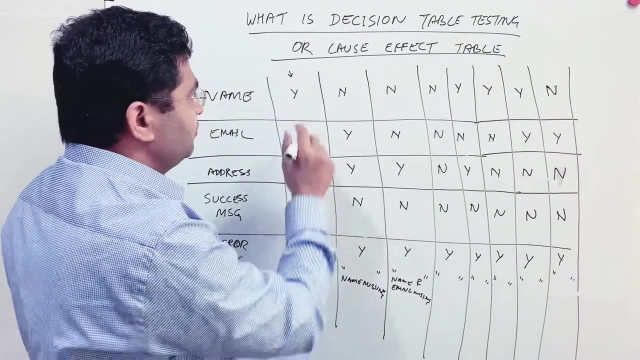 available or cause-effect table available, and what you can simply do is these all become your tests. so, in this particular case, what you can simply refer to this decision table. you will enter name and email and address and verify that the registration is getting successful. if it is getting successful, 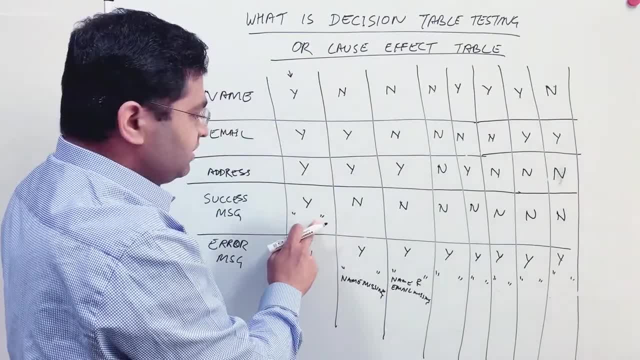 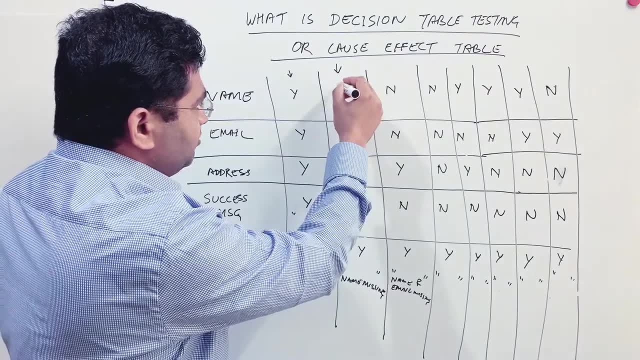 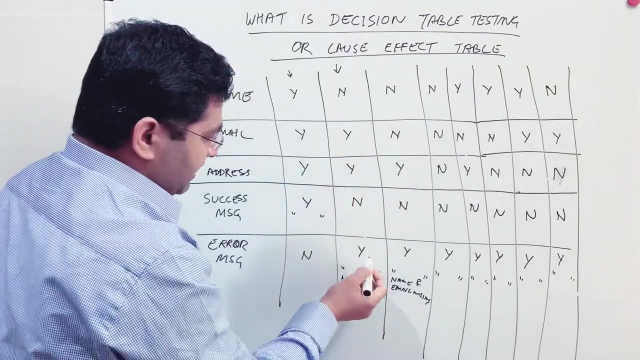 no error message successful. you know registration message. then this test is passed. this becomes your second test. in this case, you make the name and the name field as blank, provide email and address and make sure that registration fails and you get the appropriate error message. and this is. 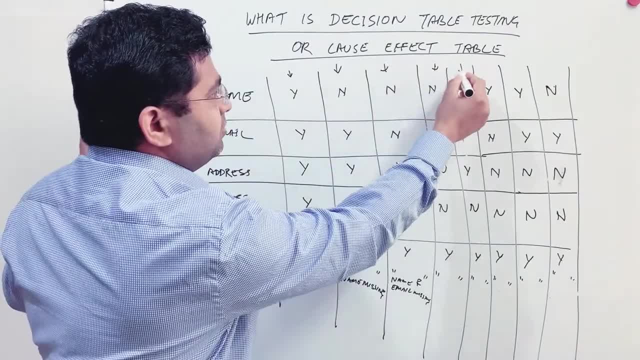 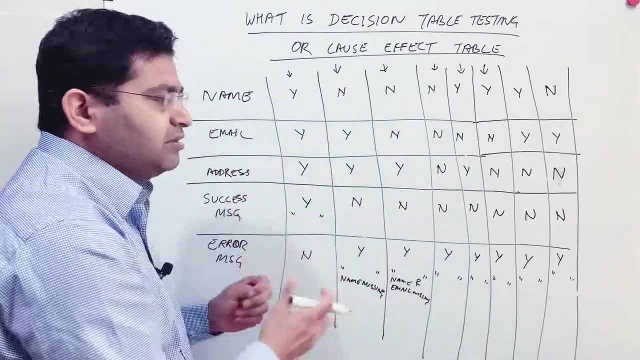 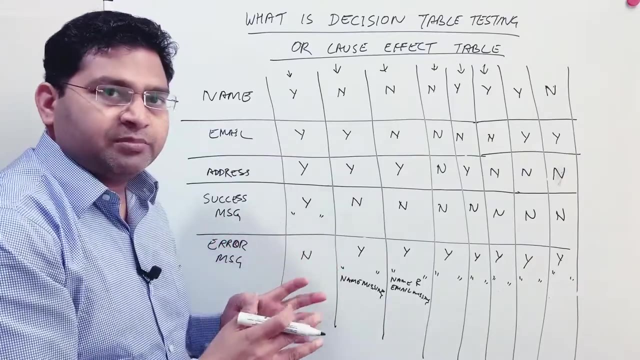 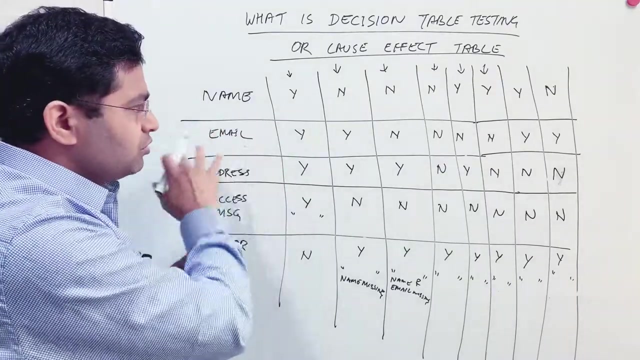 what you keep continuing with this cause-effect table or decision table to basically test different scenarios that are possible in this particular registration example. okay, so to create a decision table, decision table or cause-effect table- you simply have to get the details of what the rules are, so you put them into the rows and then, based on those inputs, if 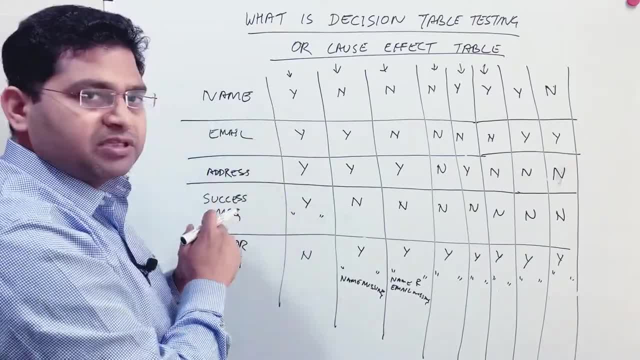 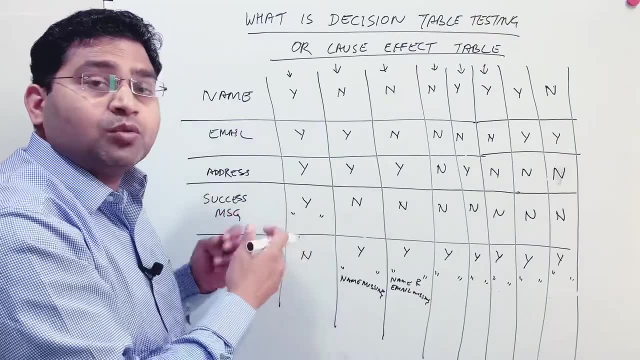 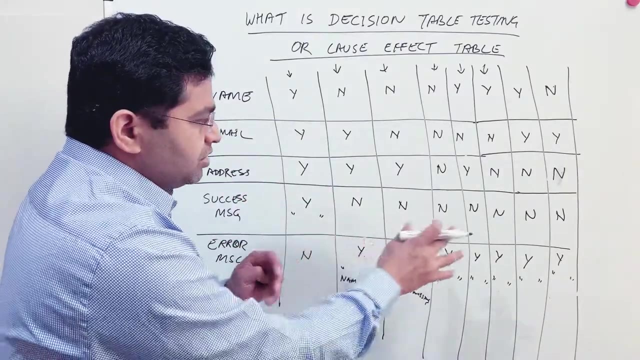 say, for example: first input is present, the second is not present, third is not present. based on those inputs, you define what will be the what is the required output based on the requirement that is defined. and once you define all these output based on the requirement, these are the tests that you need to perform. 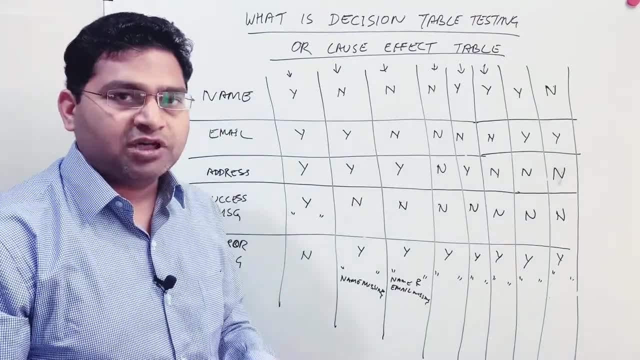 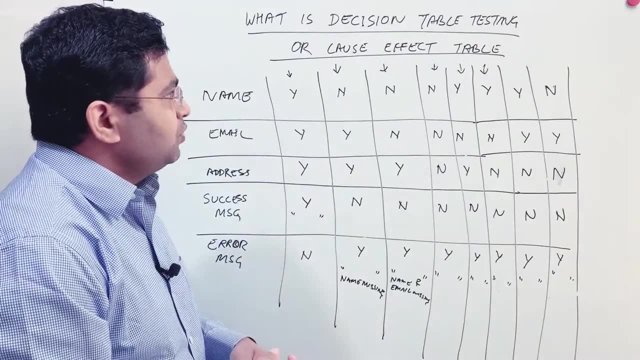 to ensure that your decision table is getting successful. so this is a very important test that you need to perform to ensure that your getting better and good coverage of the modules or the software that you are going to test. all right, so this is the simplest you know way to understand. 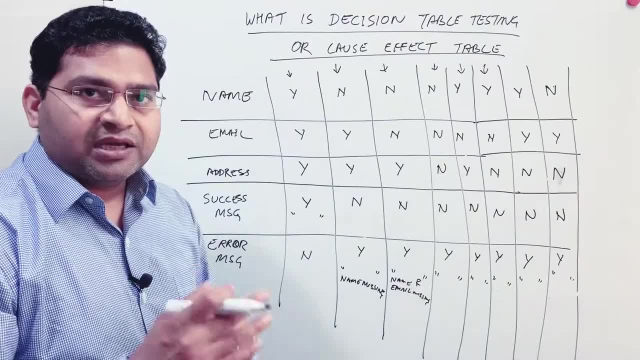 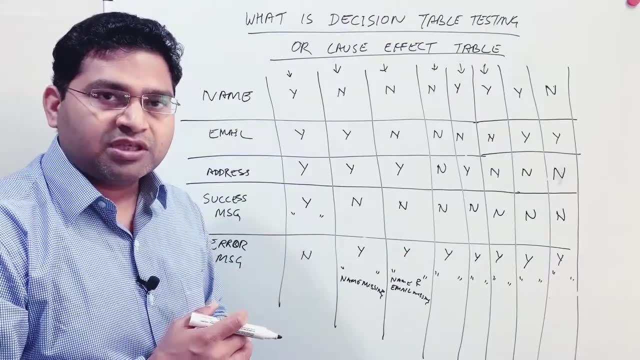 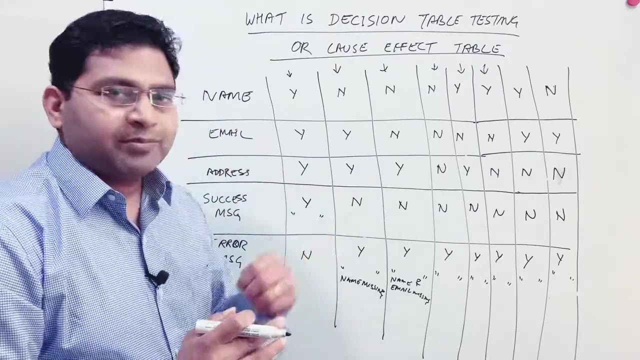 decision table testing or cause-effect table testing, and you can easily correlate this with other examples. try to you know, think of other examples that you can think of. Google around and make sure that you understand. decision table testing apply the same concept that I have explained here and 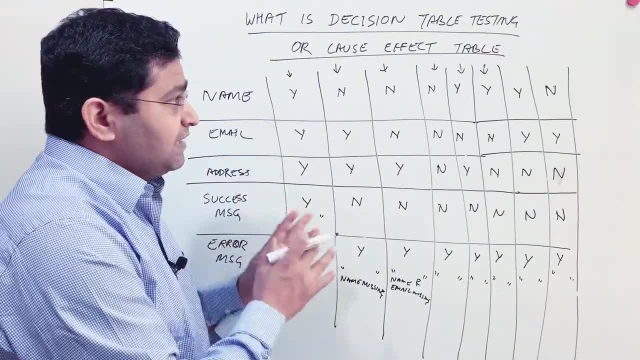 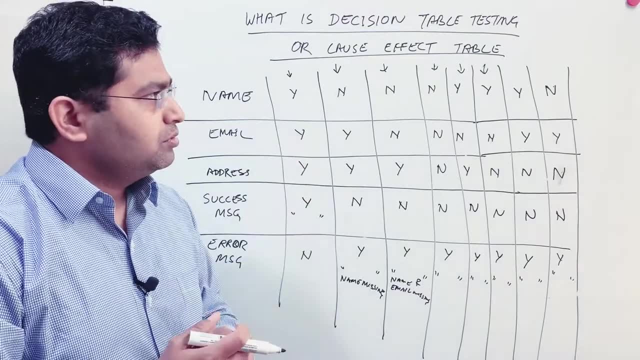 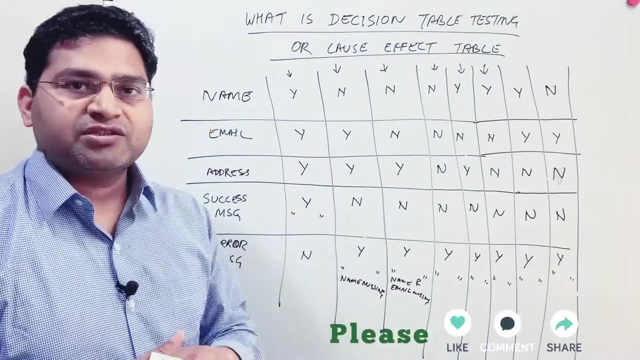 make sure that you are, you know, you understand this concept very well before you attempt or go for interview, and this will help you a lot to crack the interview as well as, basically, you know, when you get into the software testing, you will be applying these techniques to actually test the software. all right, so 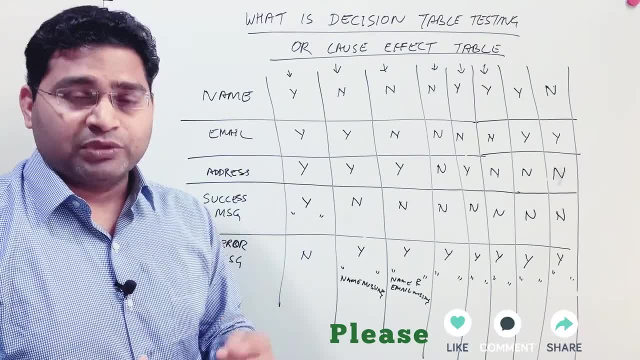 that's all for this tutorial. hope it was helpful. thank you very much for watching. 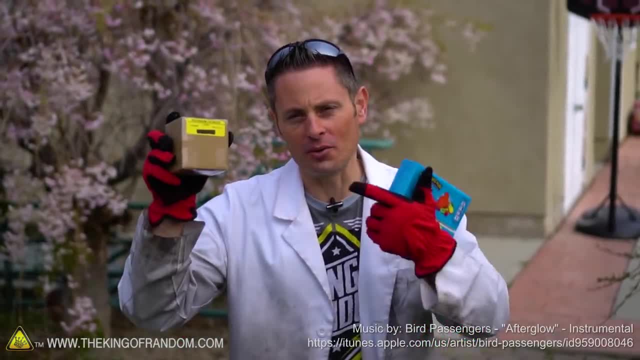 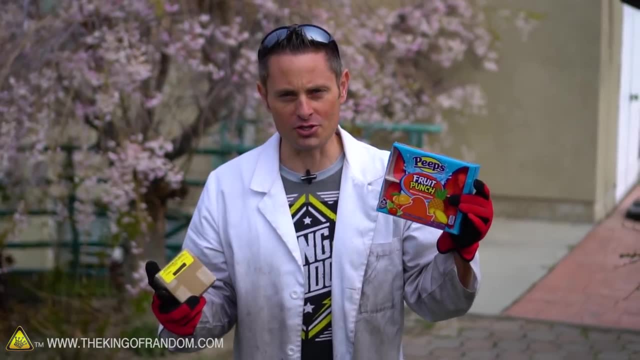 Hey guys, welcome back to the King of Random Cooking Show, where today we're cooking with a fun little chemical called potassium chlorate. Now it's that time of year where these little marshmallow peeps start popping up all around the local grocery store.